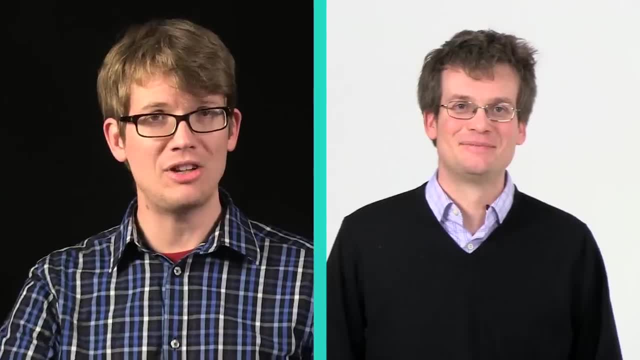 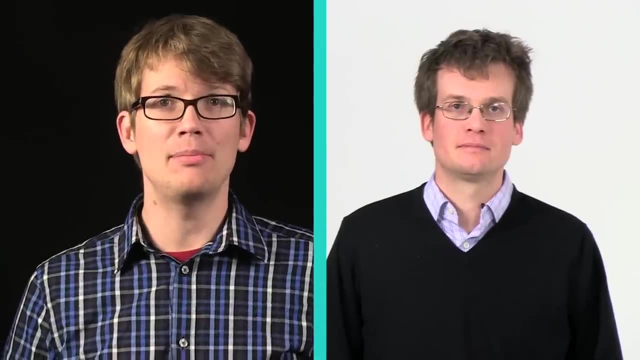 So I have this brother, John- You may have heard of him Hi there- And, as it happens, John and I have the exact same parents- Yes, Mom and Dad Green- And since we have the same parents, it's to be expected that John and I would have similar physical characteristics. 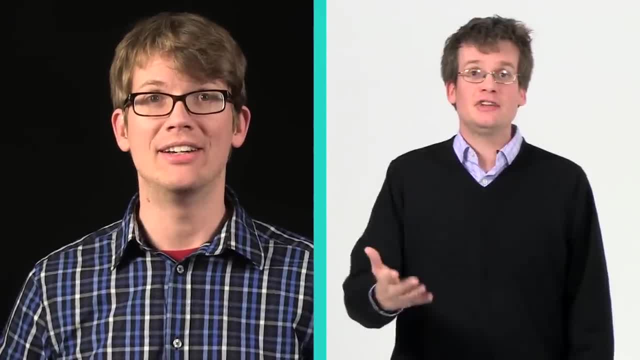 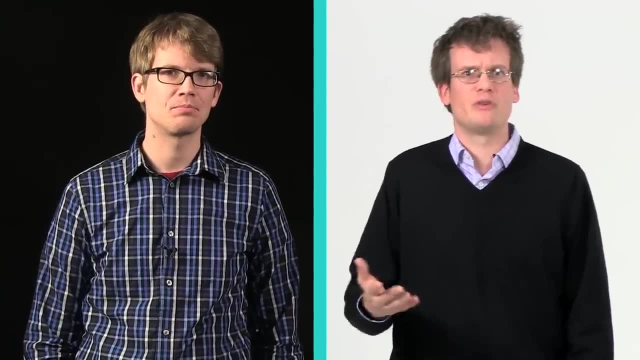 because the source of our DNA is exactly the same. Hank and I share some genes, but no one knew anything about chromosomes or DNA until like the middle of the 20th century, and people have been noticing that brothers tend to look alike since, like people started noticing stuff or whatever. 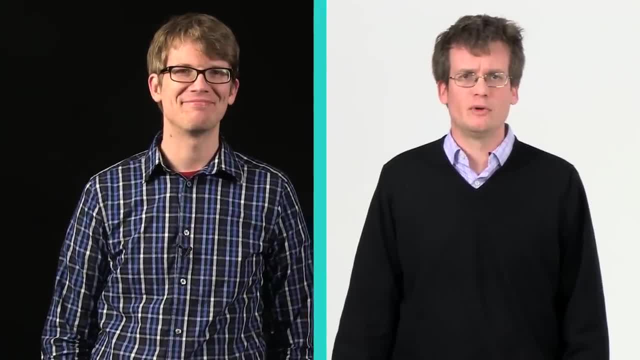 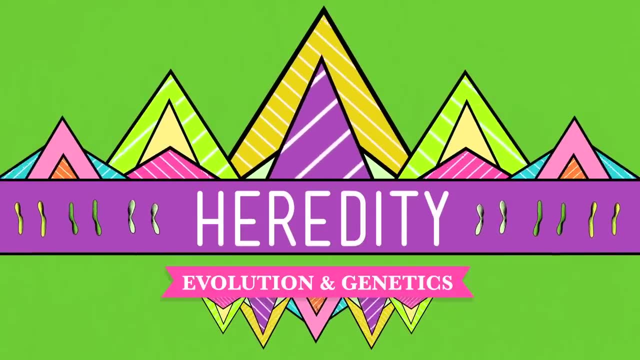 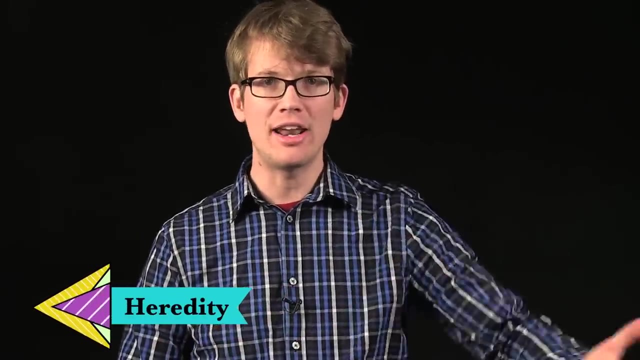 That's very scientific, John. I will remind you that I am doing you a favor. Heredity, It's basically just the passing on of genetic traits from parents to offspring And, like John said, the study of heredity is ancient, although the first ideas about how the goods were passed on from parents to kids 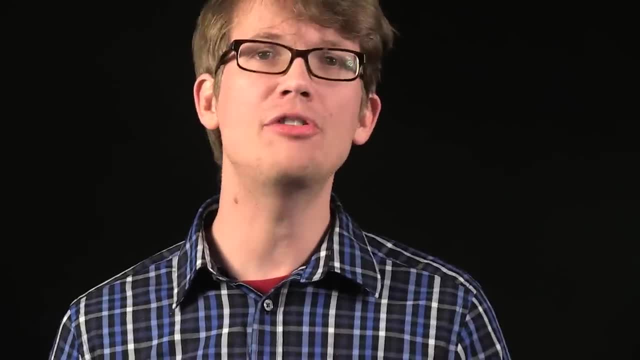 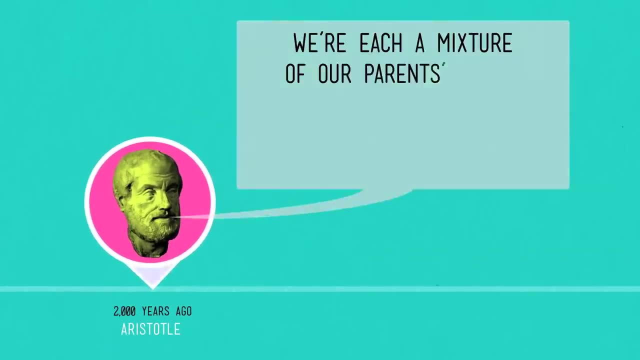 were really really, really, really, really, really wrong. For instance, the concept that people were working with for nearly 2,000 years came from Aristotle, who suggested that we are each a mixture of our parents' traits, with the father kind of supplying the life force to the new human. 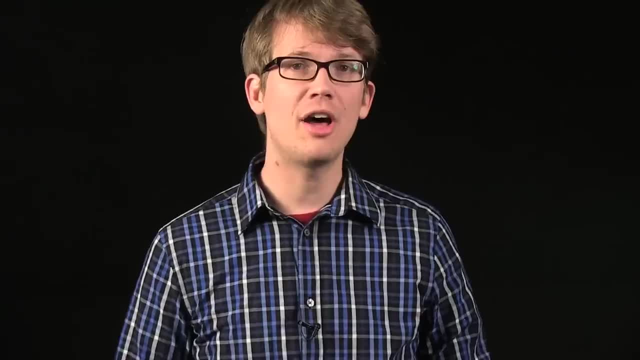 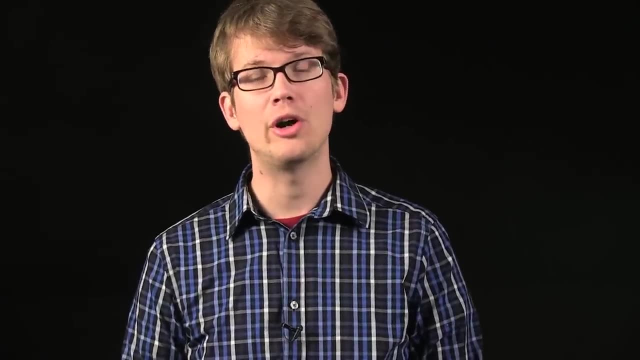 and the mother supplying the building blocks. to put it all together, Aristotle also thought that semen was like highly purified menstrual blood, which is why we still refer to bloodlines when we're talking about heredity. Anyway, since nobody had a better idea and since nobody really wanted to tangle with Aristotle, 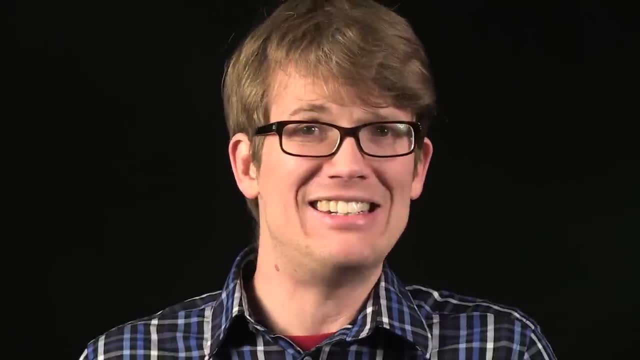 for hundreds of years everybody just assumed that our parents' traits just sort of blended together in us like of a black squirrel and a white squirrel. If a white squirrel fell in love and decided to start a family together, their offspring would be gray. 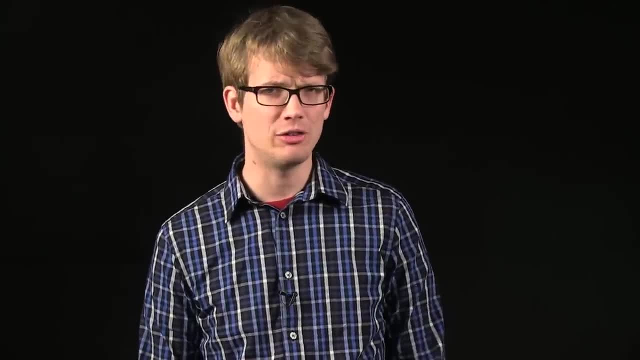 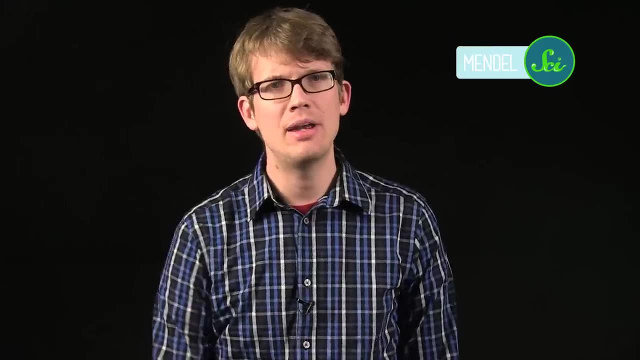 The first person to really start studying and thinking about heredity in a modern way was this Austrian monk named Gregor Mendel, And Mendel demonstrated that inheritance followed particular patterns. In the mid-1800s, Mendel spent sort of an unhealthy amount of time grubbing around in his garden with a bunch of pea plants. 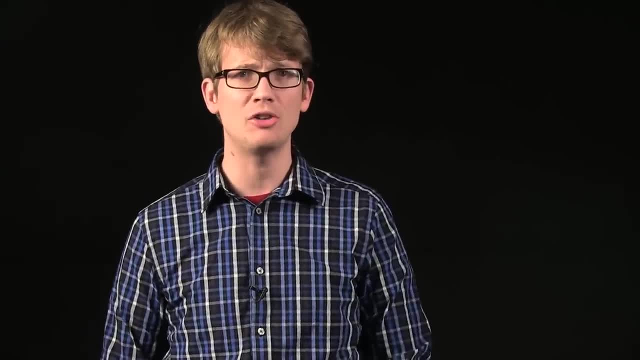 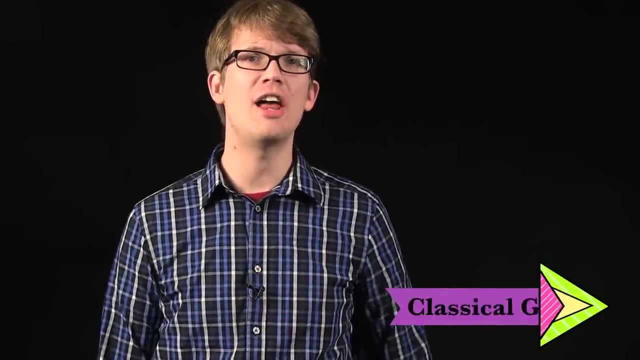 And through a series of experiments crossing the pea plants and seeing which traits got passed on and which didn't, he came up with a framework for understanding how traits actually get passed from one generation to another. So to talk about classical genetics, which includes Mendel's ideas about how traits get passed along from parents to children, 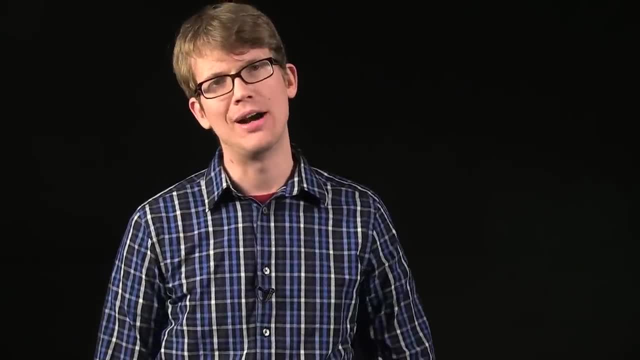 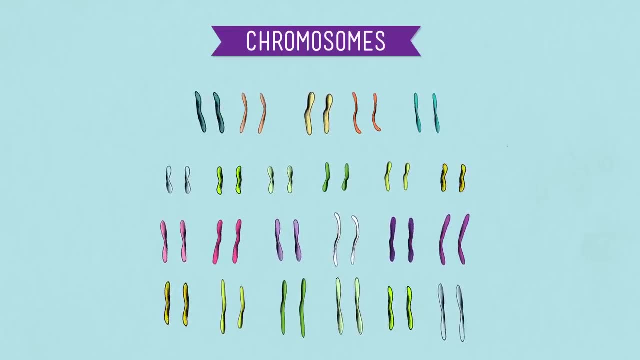 you kinda have to simplify the crap out of genetics. I hope you don't mind. So we've all got chromosomes, which are the form that our DNA takes in order to get passed on from parent to child. Human cells have 23 pairs of chromosomes. 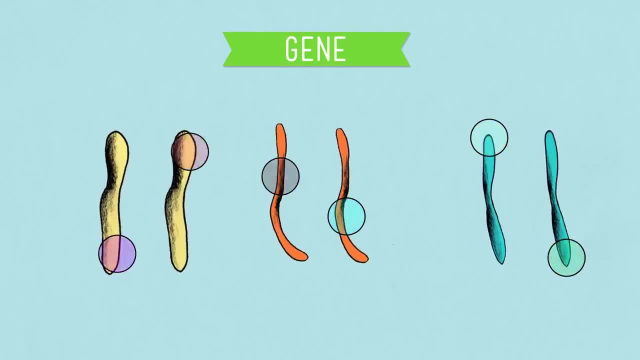 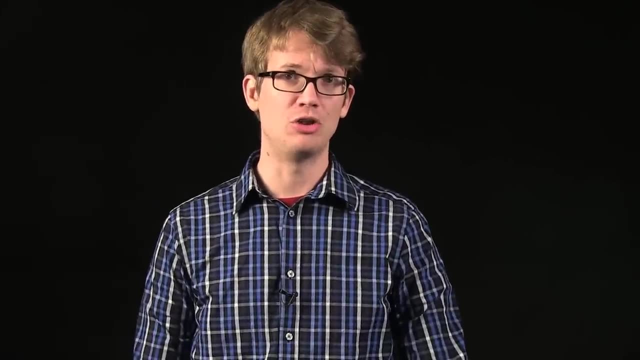 Now, a gene is a section of DNA in a specific location on a chromosome that contains information that determines a trait. Of course, the vast majority of the time, a physical trait is a reflection of a bunch of different genes working together, which makes this all very confusing. 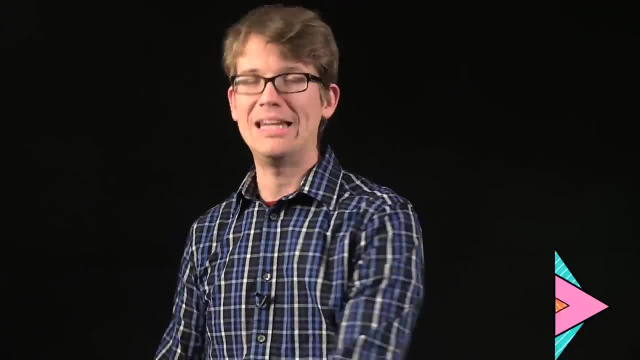 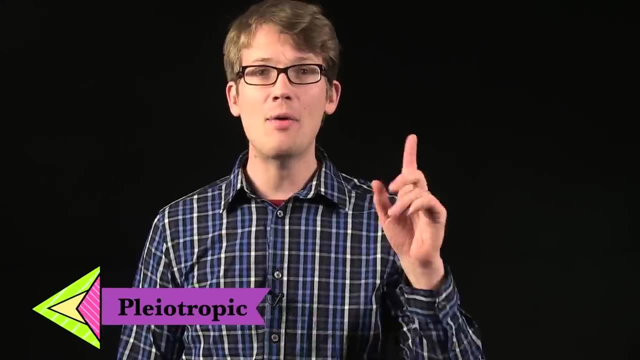 And when this happens it's called a polygenic trait, Polygenic, Many genes And then again sometimes a single gene can influence how multiple traits are going to be expressed, and these genes are called pleiotropic. However, some very few, but some single traits are decided by a single gene. 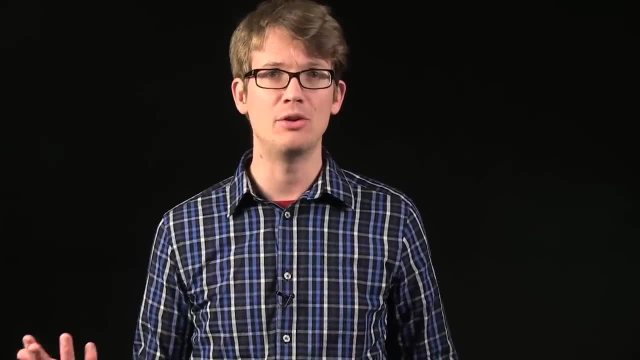 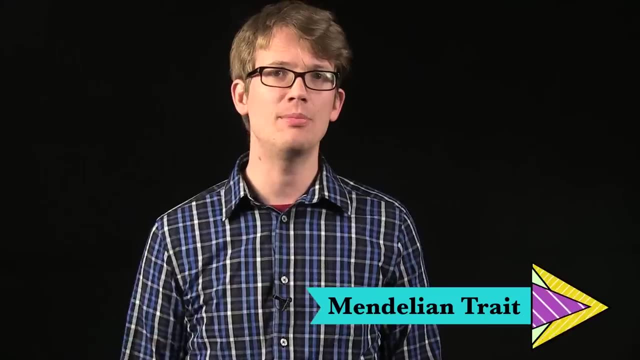 like the color of pea flowers, for example, which is what Mendel studied when he discovered all of this stuff, And when that happens in Mendel's honor, we call that a Mendelian trait. There are a couple examples of Mendelian traits in humans. 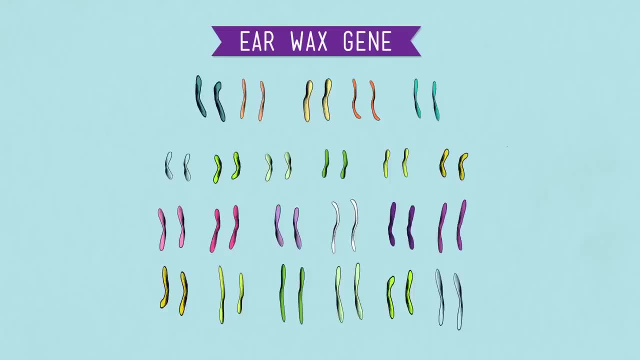 one of them being the relative wetness or dryness of your earwax. So there is just one gene that determines the consistency of your earwax, and that gene is located at the very same spot on each person's chromosome, right here, chromosome 16.. 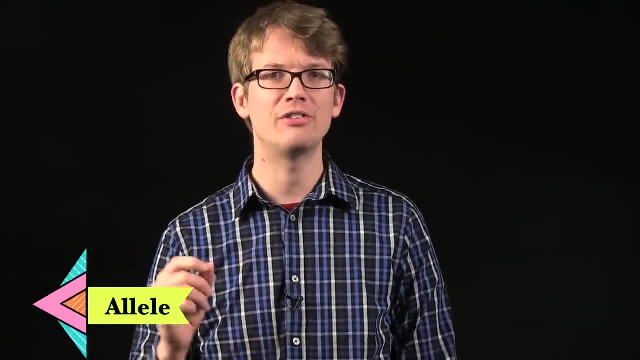 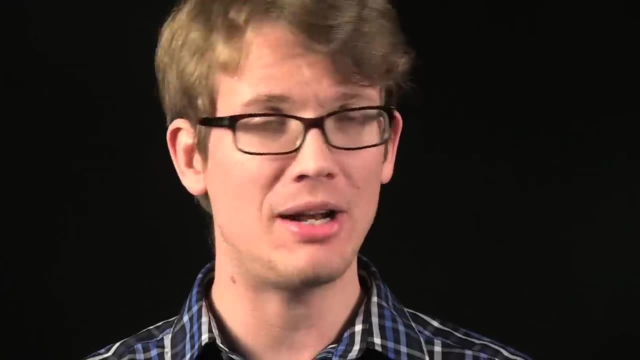 However, there's one version of this gene or allele that says the wax is going to be wet and there's another allele that says the wax is going to be dry. You may be asking yourself what the difference is between these two things. 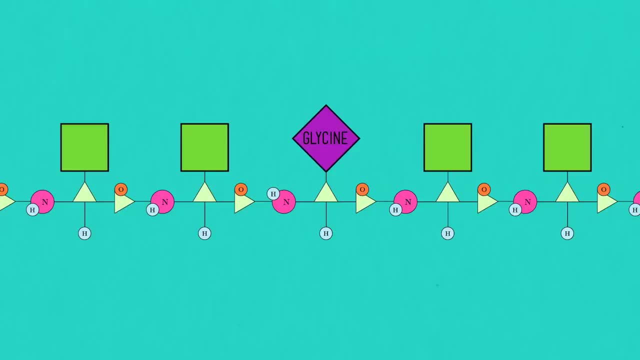 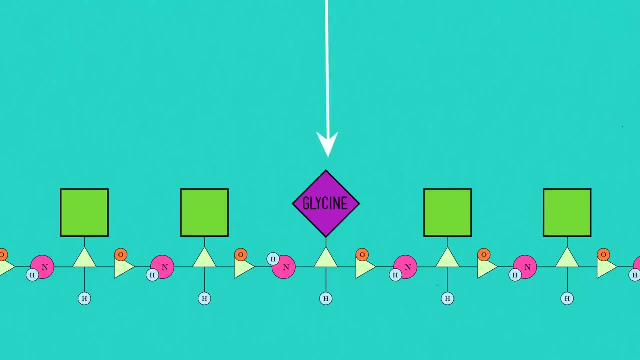 and I'm glad you asked because we actually know the answer to that question. Among the many amino acids that make up this particular gene sequence, there is one exact slot where they are different. If the amino acid is glycine in that slot, you're going to have wet earwax. 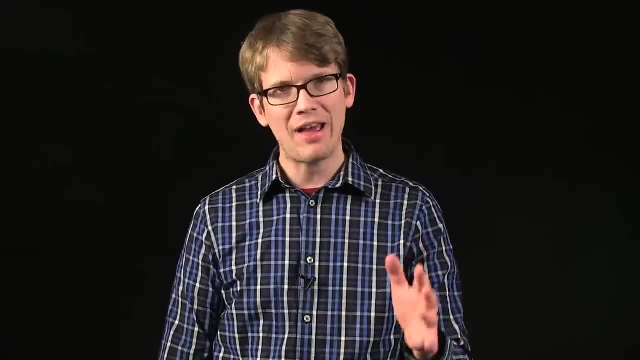 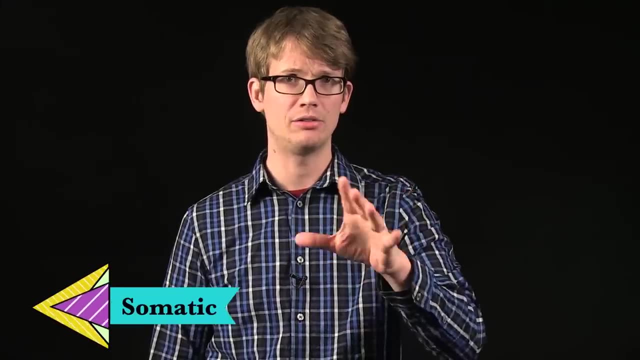 but if it's arginine it's dry. Now comes the question of how you get what you get from your parents. In most animals, basically any cell in the body that isn't a sperm or an egg- these are called somatic cells. 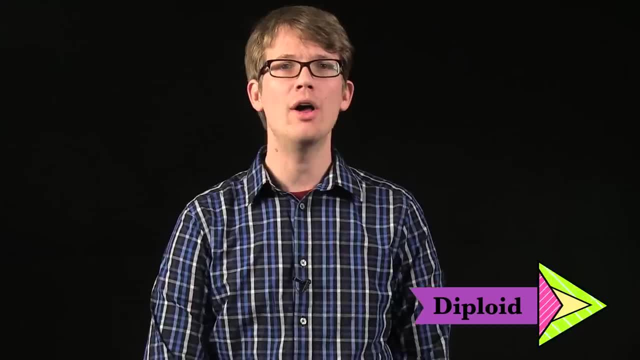 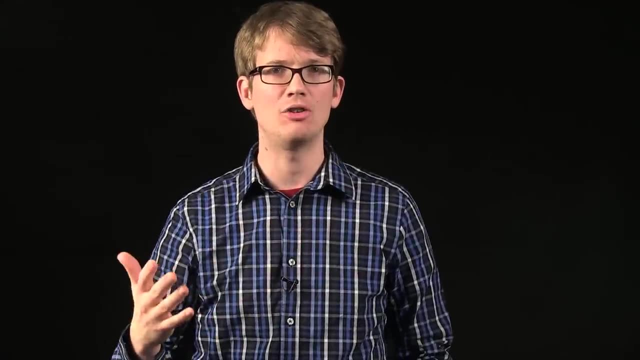 are diploid, meaning that there are two sets of chromosomes, one inherited from each of your parents. So you get one earwax-determining allele from your mom and one from your dad. And I should mention that the reason for this is that gametes, or sex cells, 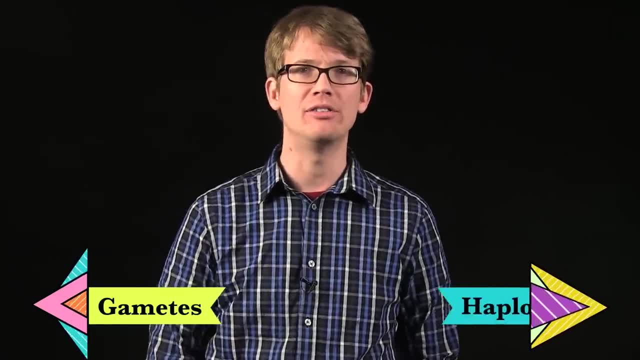 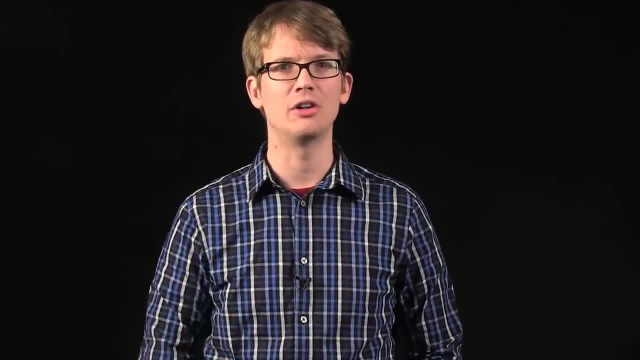 senior sperm and madame egg are haploid cells, meaning that they only have one set of chromosomes. Again for emphasis, non-sex cells are called somatic cells and they are diploid. Sex cells are called gametes and they are haploid. 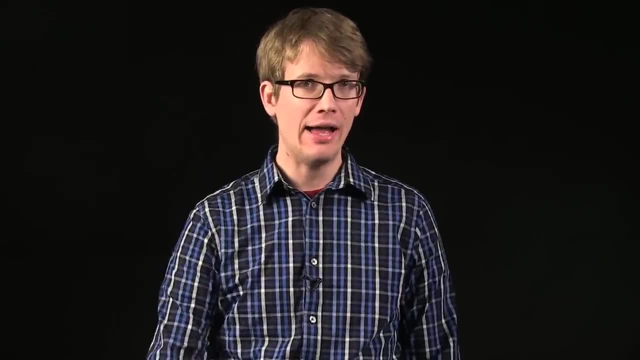 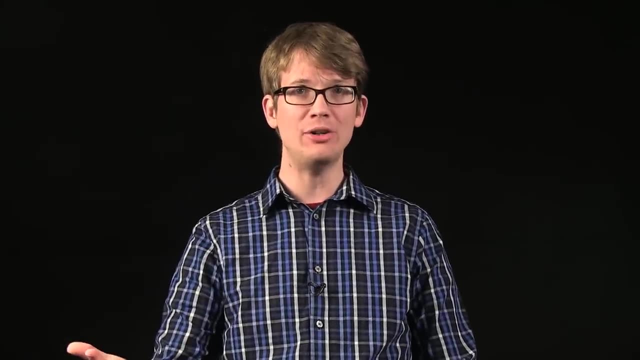 This makes a lot of sense, because a sperm or an egg has very specific motivation. They're seriously hoping to score and if they do, they plan to join with a complementary haploid cell that has the other pair of chromosomes they're going to need. to make a new human or buffalo or squid or whatever. Also, just so you know, some plants have polyploid cells, which means that they have more than two sets of chromosomes in each cell, which isn't better or anything, it's just how they do. 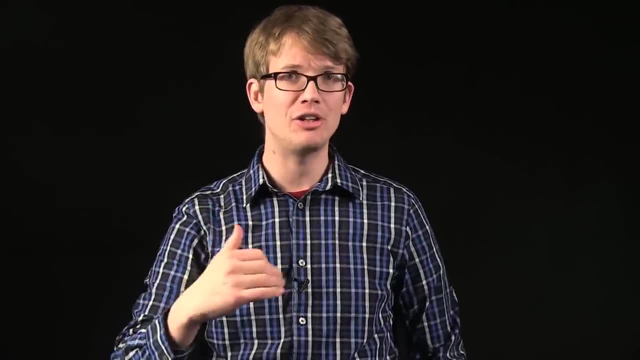 But anyway, the point of this all is that we inherit one version of the earwax gene from each of our parents. So back to earwax. So let's just say that your mom gives you a wet earwax allele. 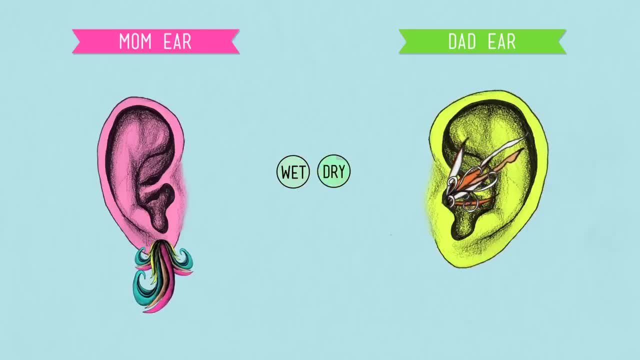 and your dad gives you a dry earwax allele. Good lord, your dad has horribly ugly ears. Anyway, since your parents have two alleles, each for one gene inherited from each of their parents, the one passed along to you is entirely random. 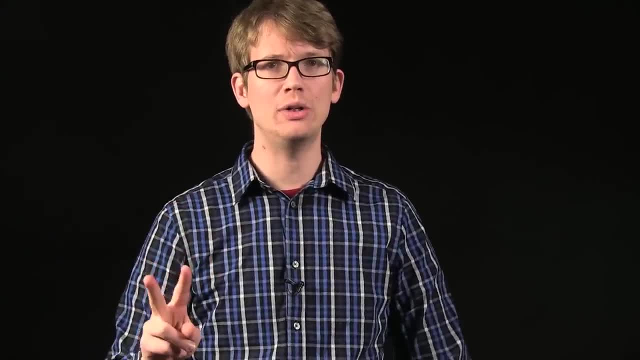 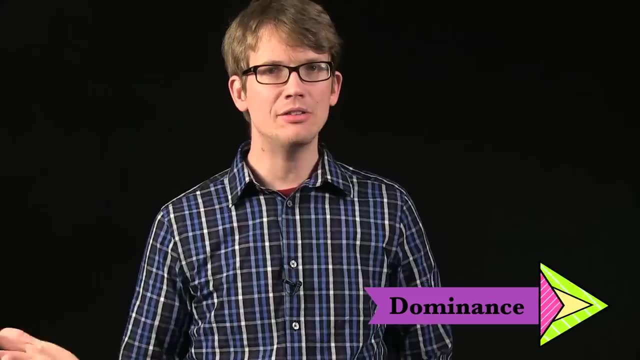 So a lot of what Mendel discovered is that when there are two alleles that decide the outcome of a specific trait, one of these alleles could be dominant and the other one recessive. Dominance is the relationship between alleles in which one allele masks or totally suppresses the expression of another allele. 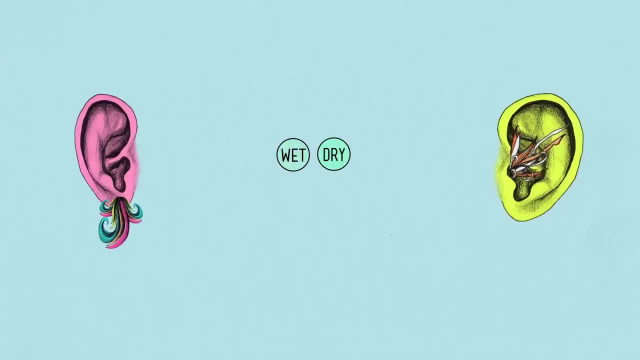 So back to earwax, because I know we all love talking about it so much. It turns out that mom's wet earwax allele is dominant, which is why she gets a big W, and dry earwax allele is recessive. 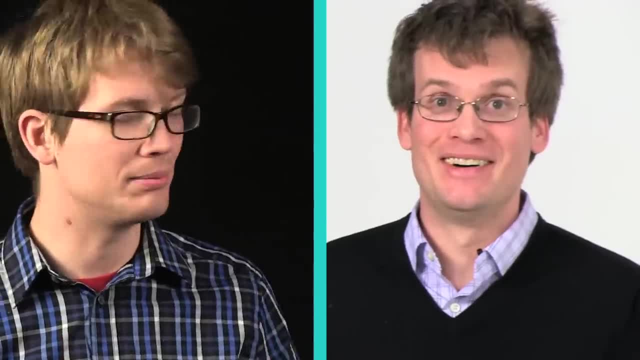 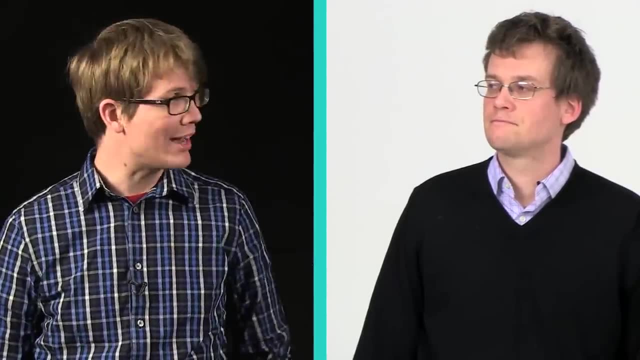 which is why he has to be a little W Go mom. Oh, you're back. Yeah, you sound surprised. Anyway, mom's allele is dominant and that settles it right. We're gonna have wet earwax. Uh, something about the way that you said that tells me it's not that easy. 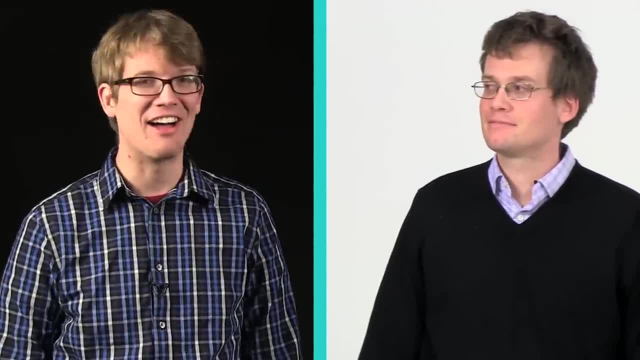 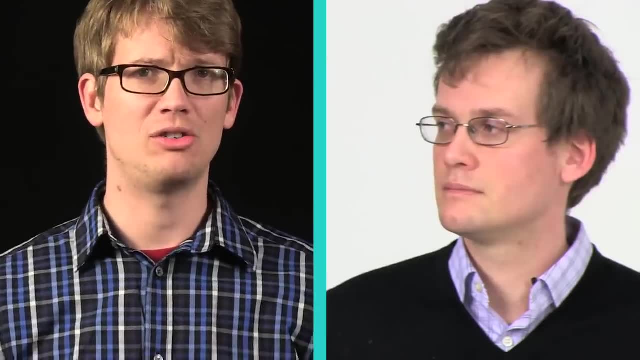 Ah, you are so much smarter than you look. It is indeed not that easy. So just because an allele is recessive doesn't mean that it's less common in all of your genetic material than the dominant allele. which leads us to the assumption, the correct assumption. 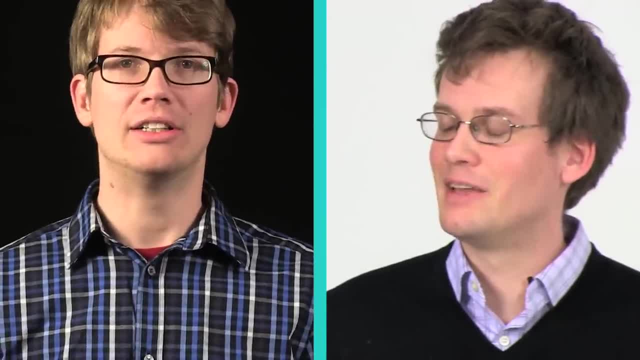 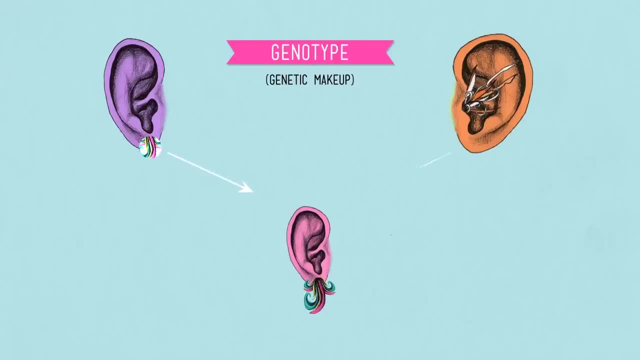 that there's something else. There's something else going on here. I'm definitely getting that vibe from you, So it has to do with mom and dad's parents, because everybody inherits two alleles from their parents. Mom got one from nanny and one from papa. 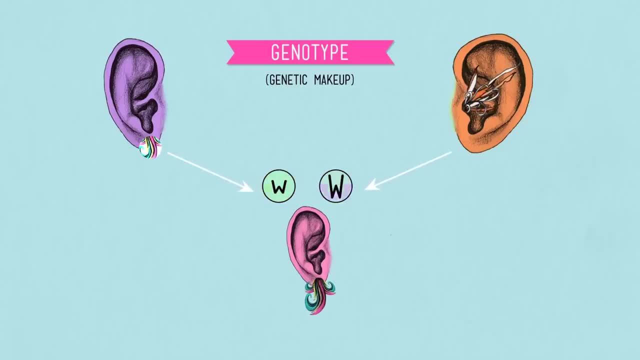 and let's just say that mom got a little W from nanny and a big W allele from papa. That means that mom's genotype or genetic makeup, when it comes to that single trait, is heterozygous, which means that she inherited two different versions of the same gene from each of her parents. 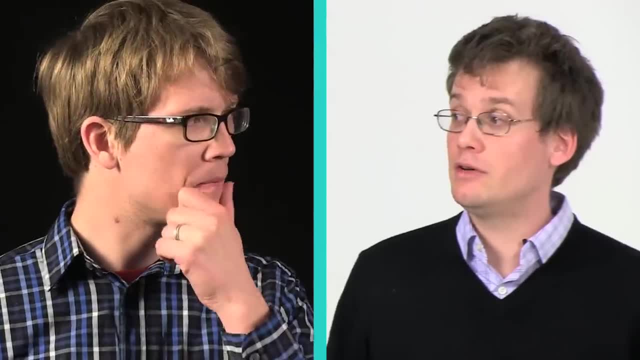 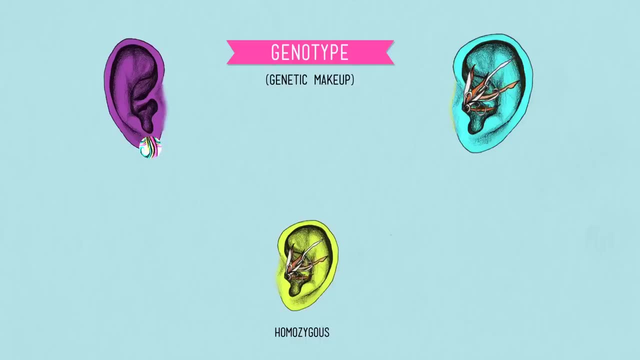 Dad, on the other hand, is a homozygote. Let me guess That means he had two of the same allele, or a little W or a big W, inherited from both grandma and grandpa Right. And in order for this to all work out the way that I want it to, 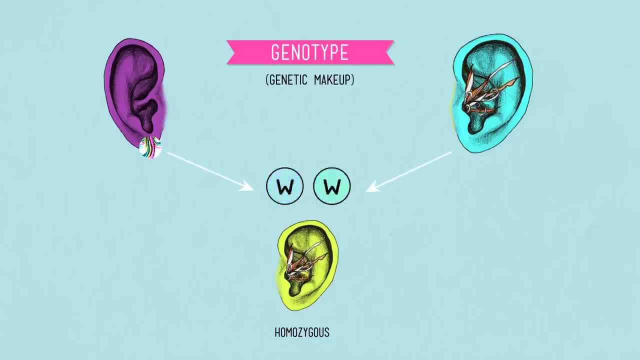 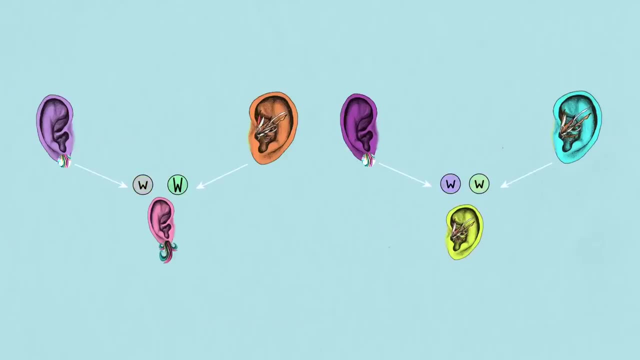 let's just say that both grandma and grandpa would have passed little Ws down to dad, making his genotype homozygous recessive for this gene. Okay, so I'm keeping score in my head right now and according to my calculations, 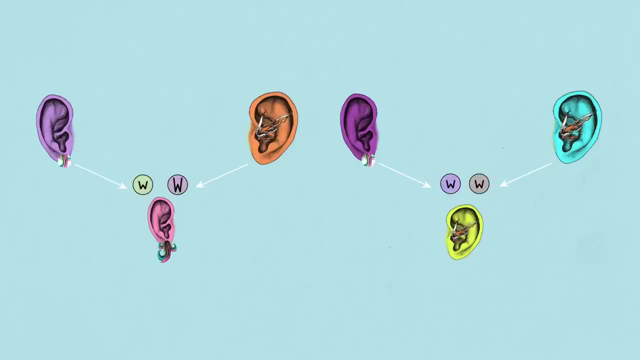 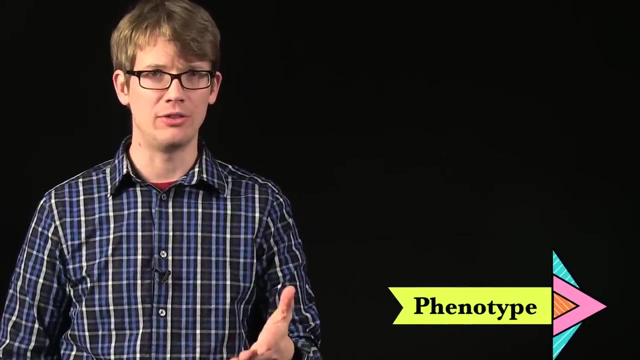 mom is a big W, little W, and dad is a little W, little W, And now we're going to try to figure out what our earwax phenotype is. And phenotype is what's expressed physically or, in this case, what you'd see if you looked into our ears. 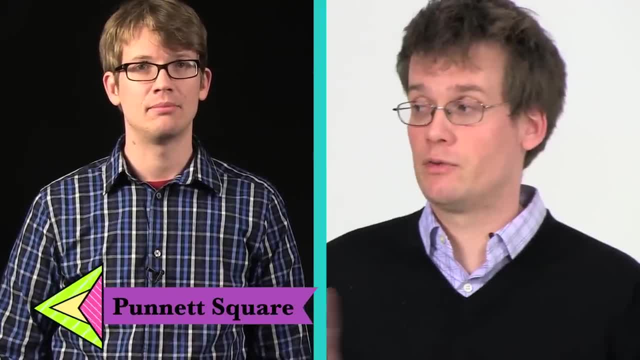 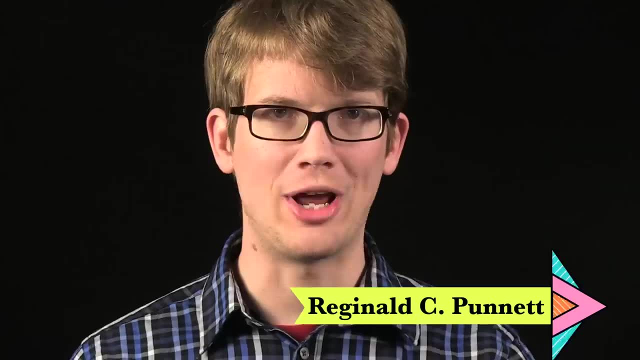 All right. so we're going to do like a Punnett square or anything. This is why I do history. If we're doing Punnett squares, I'm leaving, But I was just going to start to talk about people again. So Reginald C Punnett, who was a total Gregor Mendel fanboy. 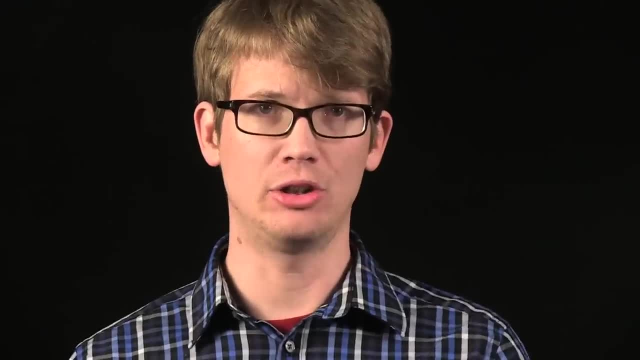 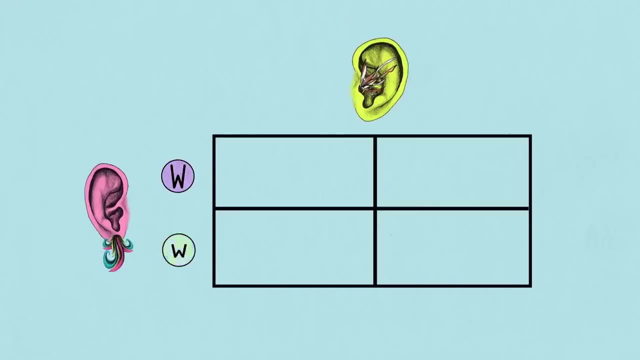 invented the Punnett square as a way to diagram the outcome of a particular crossbreeding experiment, And a really simple one looks like this. So let's put mom on side here and give her a big W and a little W, and let's put dad at the top and he gets two little Ws. 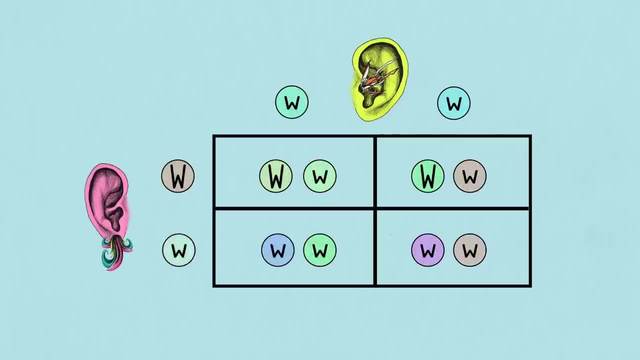 So if you fill this in, it looks like there's a 50-50 chance that any child of this mating will be homozygous or heterozygous. And as for our phenotype shakes out the same way, John and I both have a 50% chance of having wet earwax. 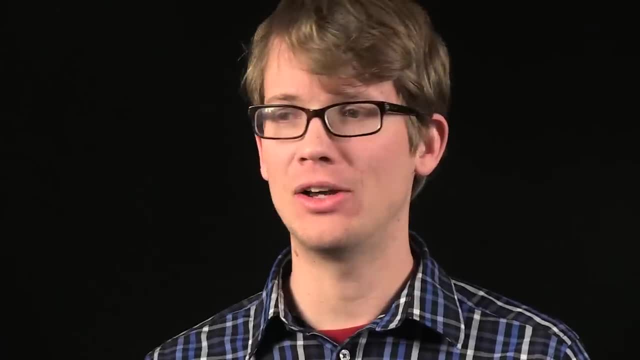 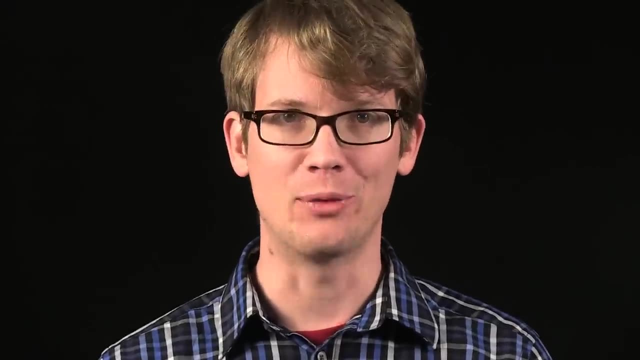 a 50% chance of having dry earwax. So I just had to go and call John, because now he's not participating, because he doesn't like Punnett squares, And it turns out that he has wet earwax. I also have wet earwax. 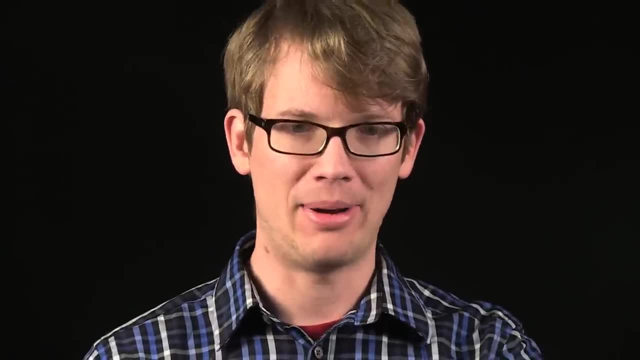 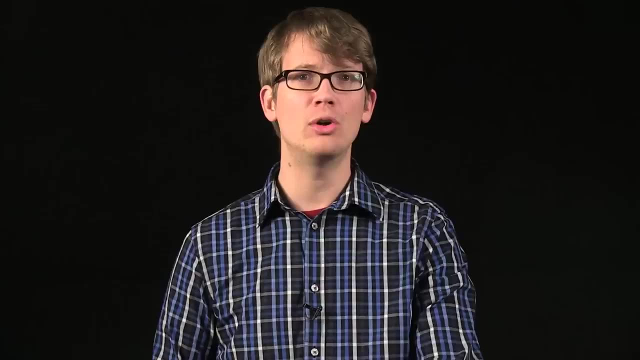 which you know is not that unlikely, considering that our parents were homozygous and heterozygous. This may explain the odor of our bed. We were in the bathroom when we were growing up, because it turns out that there's a correlation. 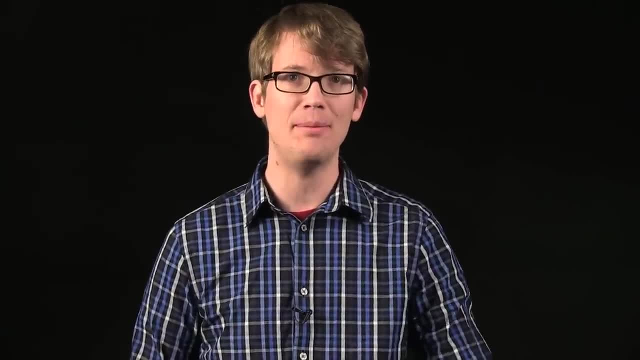 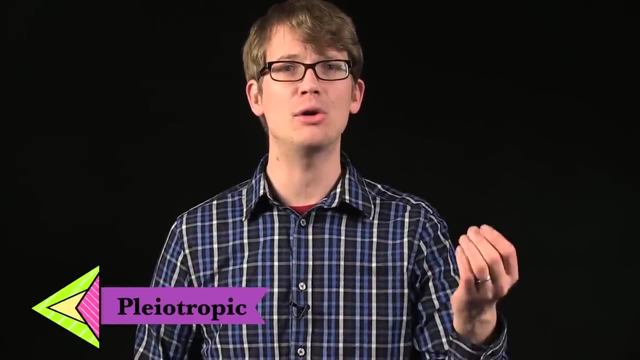 between wet earwax and body odor, because earwax and armpit sweat are produced by the same type of gland. Because this one gene has an effect on multiple traits or phenotypes. it's an example of a pleiotropic gene, because the gene affects both how wet your earwax is. 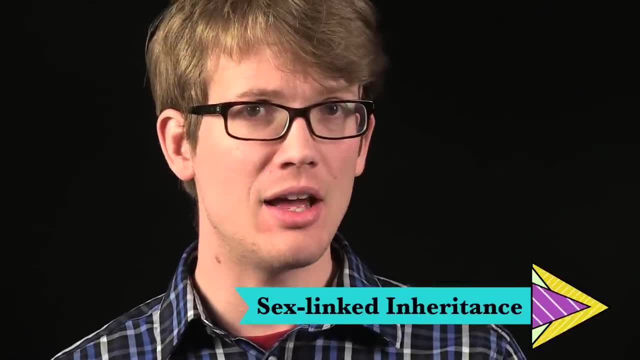 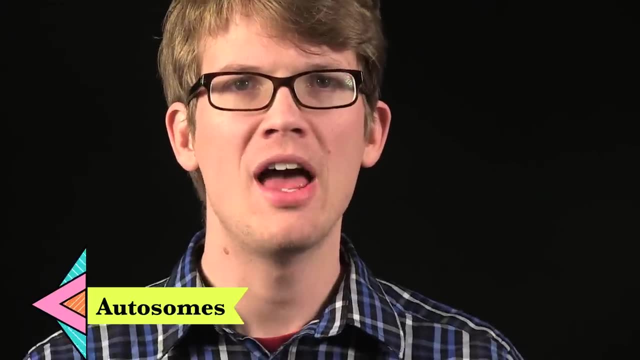 and how much you stink. One more thing you might find interesting: sex-linked inheritance. So we've got 23 chromosomes. 22 pairs are autosomes or non-sex chromosomes and one pair, the 23rd pair, to be exact. 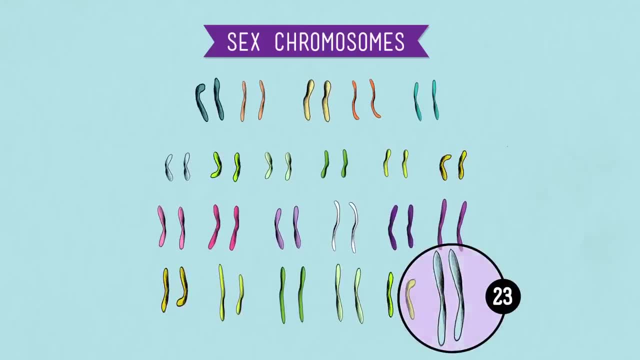 is a sex chromosome. At that 23rd pair, women have two full-length chromosomes, or XX, and men have one X chromosome that they inherited from their mom and this one little short, puny, shriveled chromosome that we call Y. 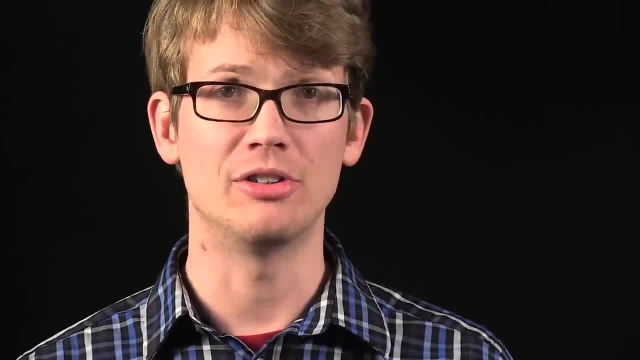 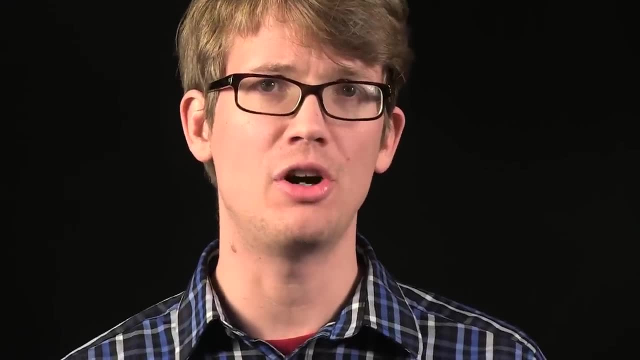 which is why men are XY. So certain genetic traits are linked to a person's sex and are passed on through the sex chromosomes. Since dudes don't have two full chromosomes on pair 23, there may be recessive alleles on the X that they inherited from their mom. 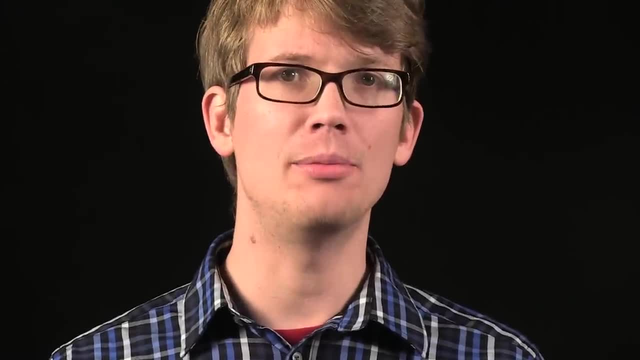 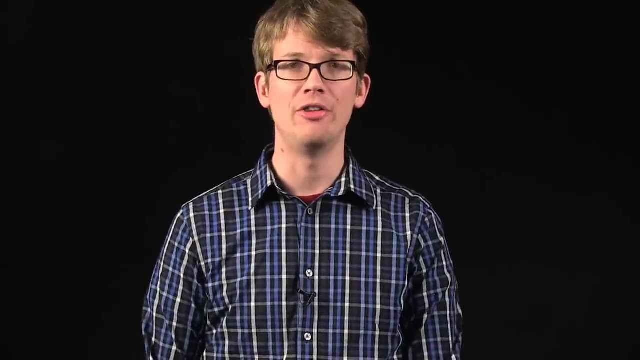 that will get expressed, Since there's not any information on the Y chromosome to provide the possibility for a dominant allele counteracting that specific trait. Take, for instance, balding Women rarely go bald in their youth, like some men do, because it's caused by a recessive allele. 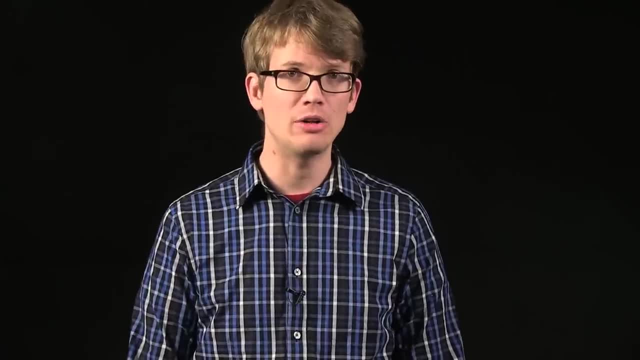 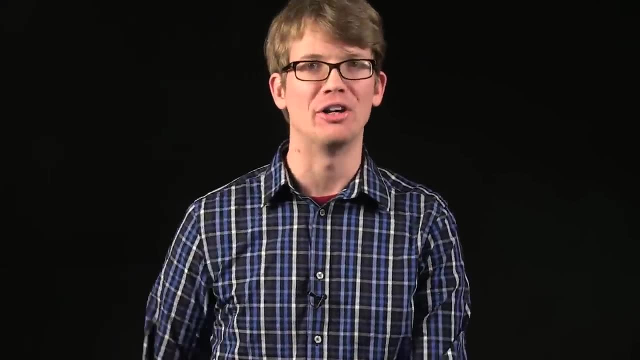 located in a gene on the X chromosome. So it's rare that women get two recessive alleles. but men need just one recessive allele and don't baldy bald. And that allele is on their X chromosome, which they got from mom. But was mom bald? 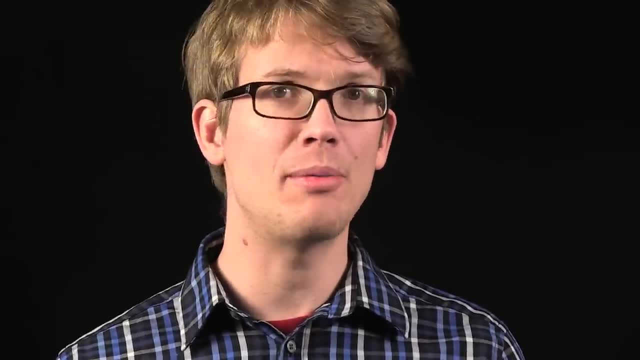 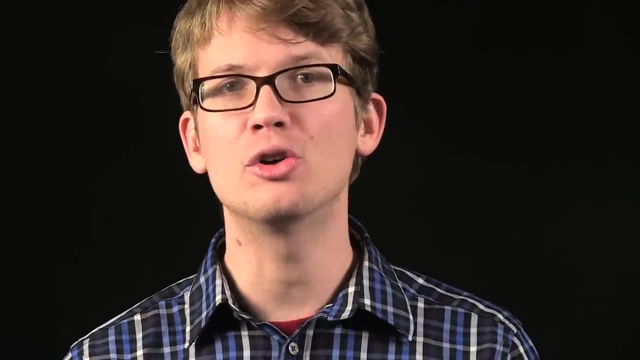 Probably not. And where did mom get that allele on her X chromosome? Either from her dad or her mom. So if you're bald, you can go ahead and blame it on your maternal grandmother or your maternal maternal great grandfather or your maternal maternal maternal great great grandfather. 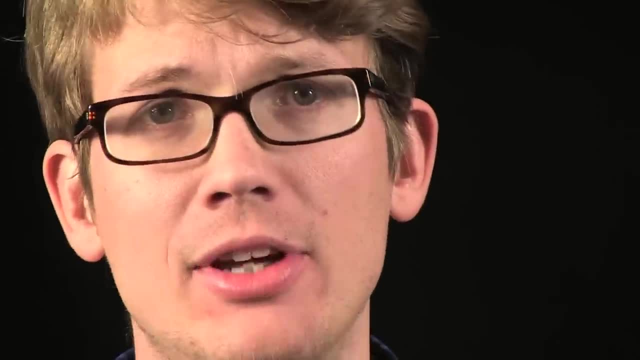 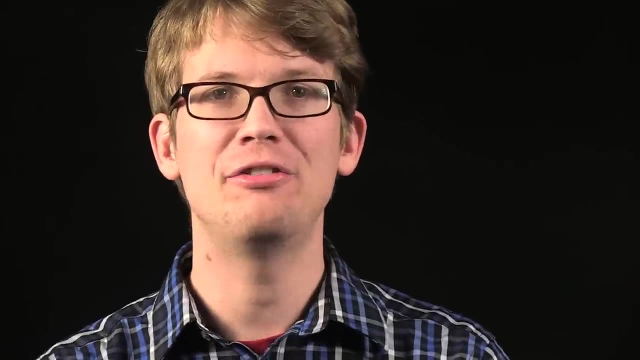 who probably went bald before he was 30. So genetics, you guys, Resistance is futile. Thanks to my brother, John, for sharing his personal genetic information with us, and also his face and voice and all of that stuff. That was very nice. 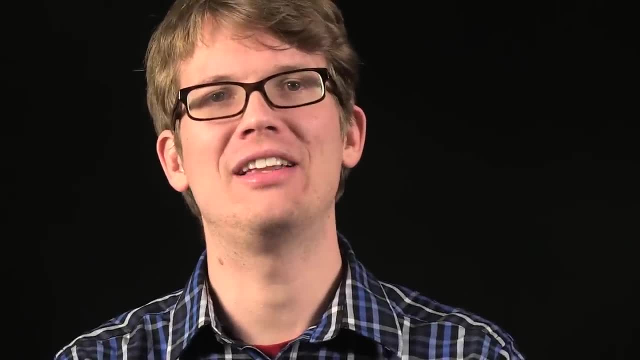 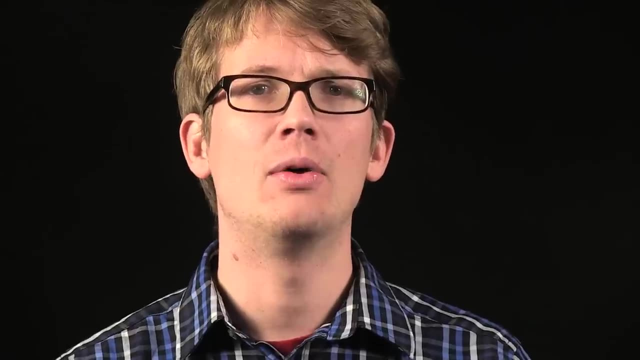 And think of us next time you swab out your ears. Actually, they say that you really shouldn't do that, because you have earwax for a reason and you might poke your brain or something. Okay, That's the last time I'm mentioning earwax. 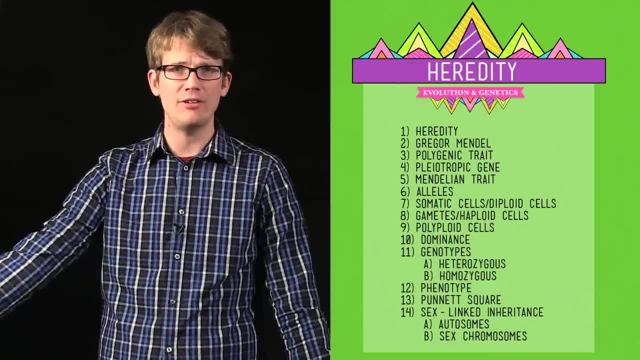 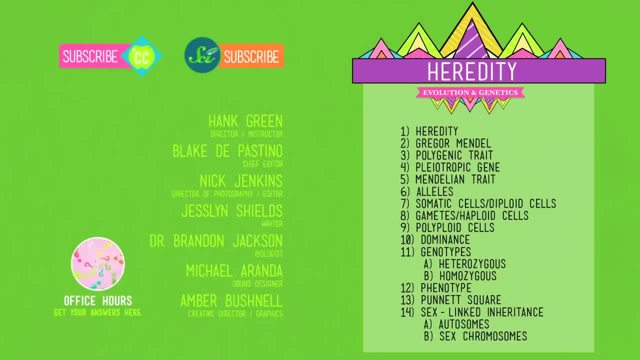 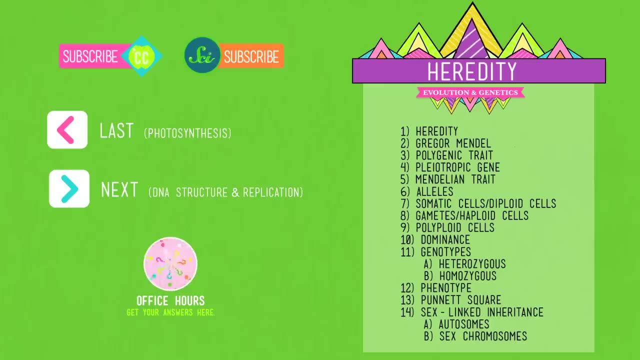 Review. Click on any of these things Back to that section of the video. If you have any questions, please ask them in the comments, Thank you. Thank you for watching. If you haven't subscribed yet, please do so right away. and also, if it's not already done, I have a job bingo coming up Like this0 and this Head over ser Fund: overcome helipad and try families.